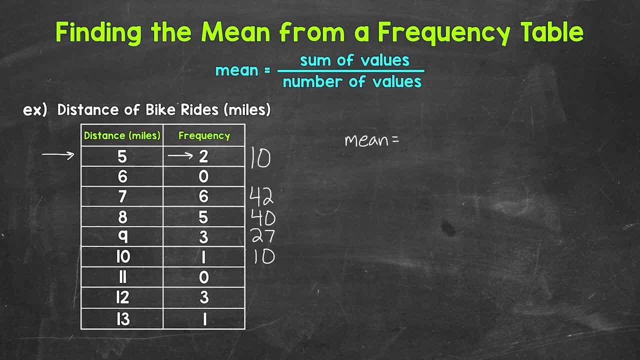 at all, So we don't need any elevens. Then twelve miles occurred three times times- that gives us 36- and then 13 miles occurred once. So again, instead of writing out each individual value, we can use the frequency table to combine values. Then we can write out an addition. 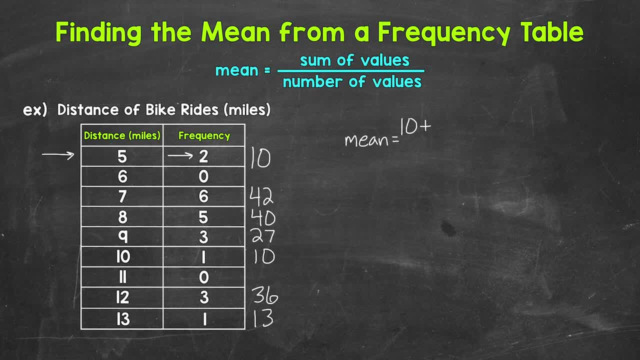 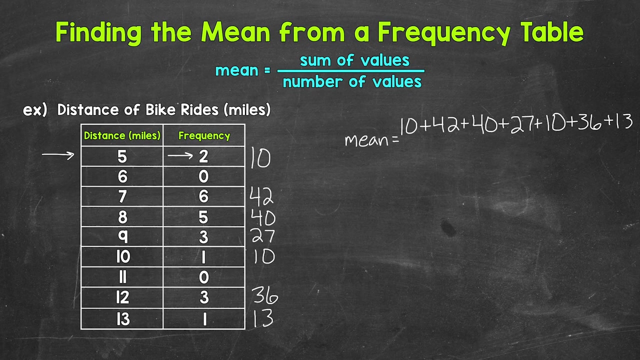 problem here. So we have 10 plus 42 plus 40 plus 27 plus 10 plus 36 plus 13.. So that's going to give us the sum of all of the values, the total number of miles, and then we divide that by the number. 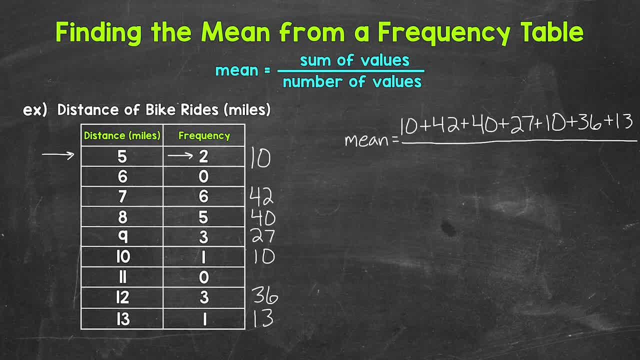 of values we have. We can look at the frequency column to figure out the number of values we have. Now we start with five miles, which occurred twice. so we have two values there. We don't have anything for six. so two plus zero is two. Then we have six values. here Seven miles occurred six. 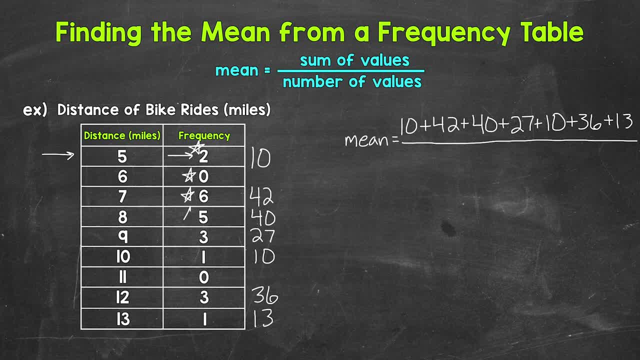 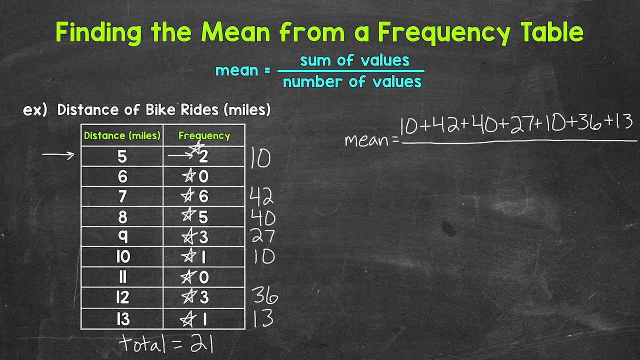 times. so two plus six is eight plus five is 13 plus three is 16 plus one is 17 plus zero. we still have 17 plus three is 20 plus one is 21.. So our total number of values is 21.. So we divide our. 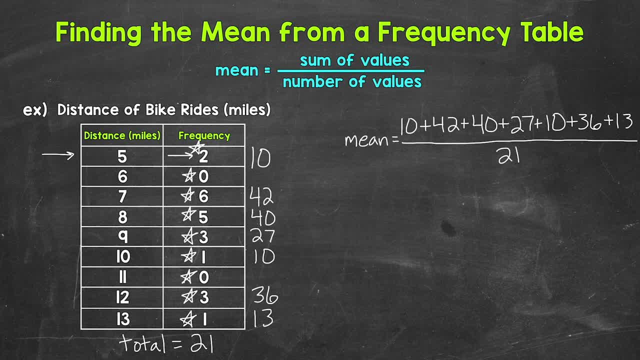 sum of the values by 21.. Now we're ready to go Add and then divide. So let's add here: 10 plus 42 is 52, plus 40 is 92, plus 27 is 119, plus 10 is 129. 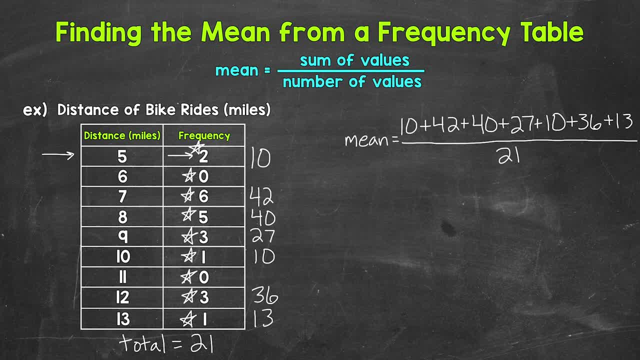 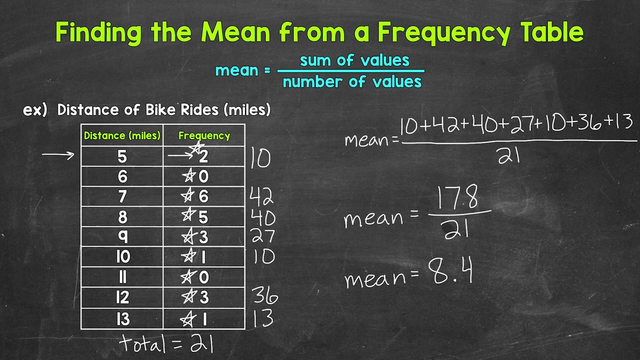 plus 36 is going to give us 165. plus 13 gives us 178. So now we have our mean is going to equal. well, the sum of our values is 178 and we need to divide that by 21.. 178 divided by 21 gives us 8.476, and that decimal